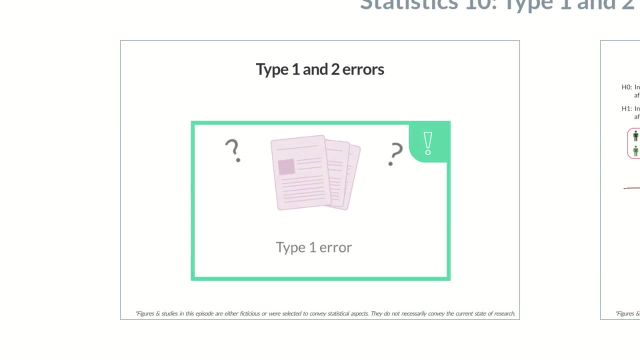 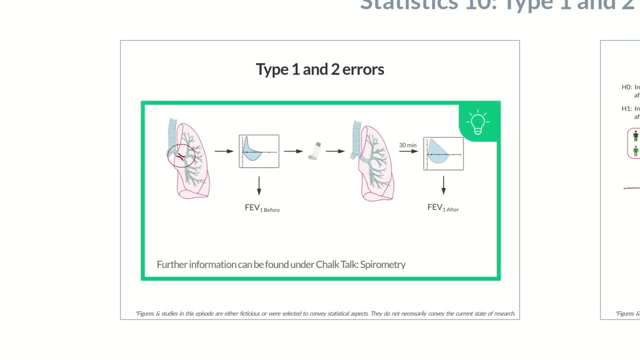 significant and non-significant findings. Let's illustrate this using the example from our last episode. A fictional study analyzed a new drug for patients with asthma. To assess its efficacy in managing bronchodilation, the patient's FEV1 value was measured by pulmonary function testing. 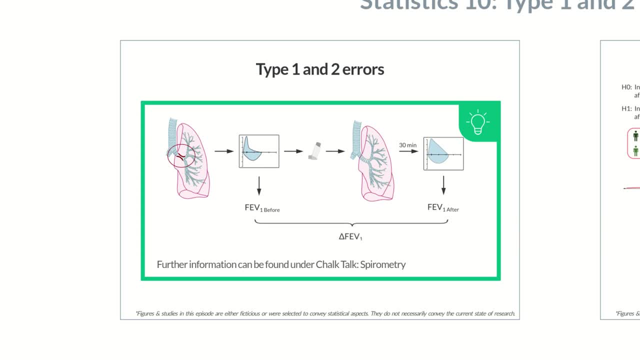 before and 30 minutes after administration of the drug. From the difference between the two values, the change in the volume of forcibly expired air in one second was determined, allowing to extrapolate the efficacy of the bronchodilating drug. The null hypothesis. 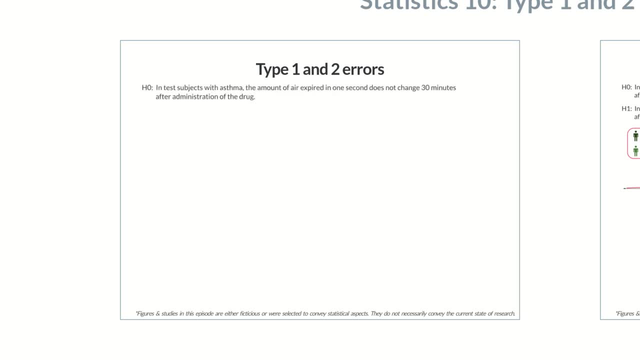 H0, to be rejected, was in test subjects with asthma. the amount of air expired in one second does not change 30 minutes after administration of the drug. The alternative hypothesis, H1,, which is mutually exclusive to the null hypothesis, was in test subjects with asthma. 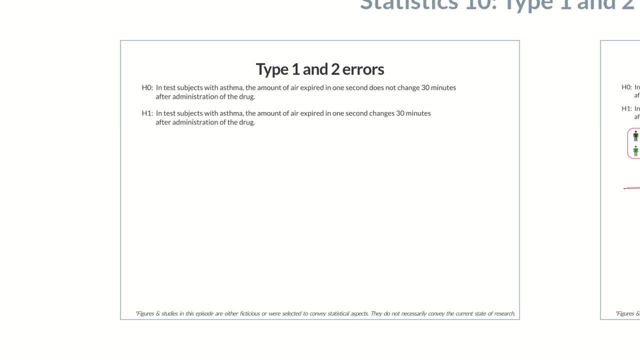 the amount of air expired in one second changes 30 minutes after administration of the drug. As we're only speaking of a general change, the hypothesis includes both positive effects, as an improvement of respiration, and negative effects, such as a deterioration. Such hypotheses are non-directional or two-tailed, because we're statistically testing both directions. 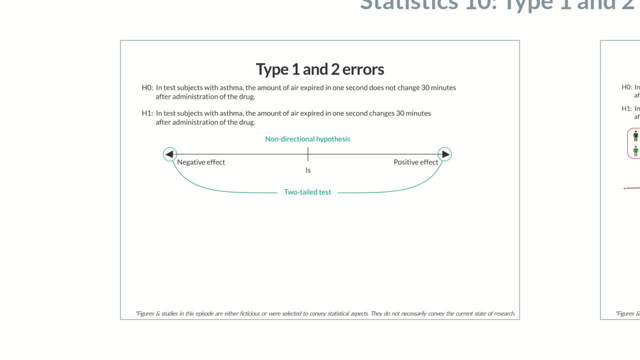 for a potential change, Had we excluded negative effects right from the start. we could have also tested the following hypothesis In test subjects with asthma: the amount of air expired in one second increases 30 minutes after administration of the drug. Then we'd only look at the results of the test subjects with asthma. 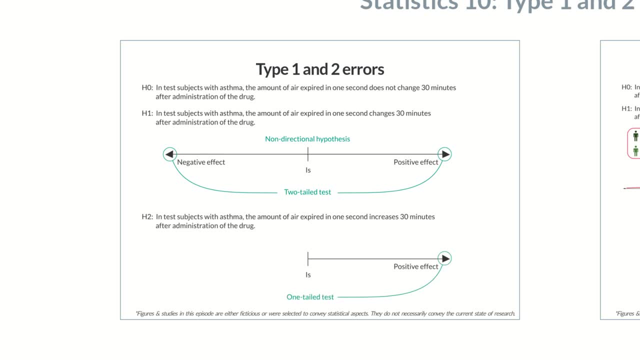 and perform a one-tailed test. Such a hypothesis is also called a directional hypothesis. However, in medical statistics analysis is usually two-tailed, so we'll show a two-tailed example here. But our fictitious example isn't a randomized controlled trial. 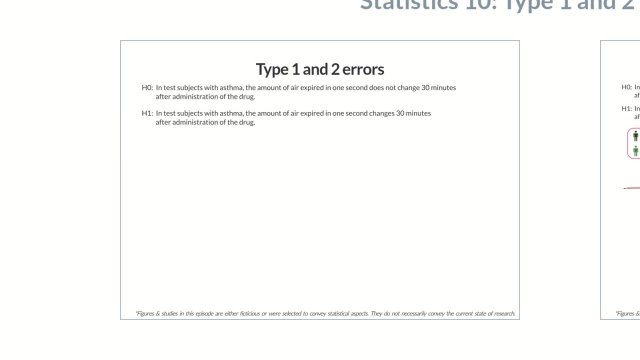 which is usually the gold standard in clinical research. In such studies, two groups are compared: an intervention group and a comparison group. But to keep things simple, here we'd like to show the statistical evaluation of a fictitious study through a simple example. So our fictitious study is testing the validity of the null hypothesis. The null 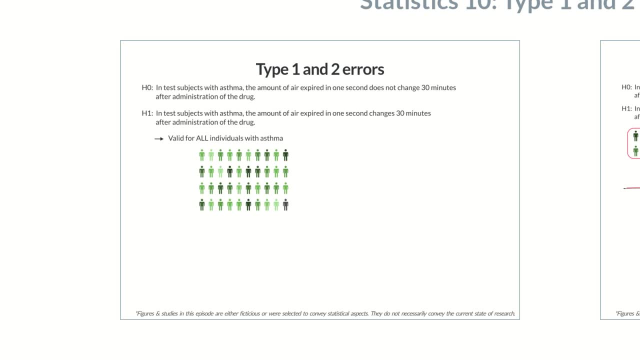 hypothesis relates to all individuals with asthma, that is, the entire population of asthmatics. However, the study obviously can't examine everyone with asthma. Therefore, a representative group is tested, known as the sample. In our example, the group comprises of two people with asthma. The group comprises of two people with asthma. 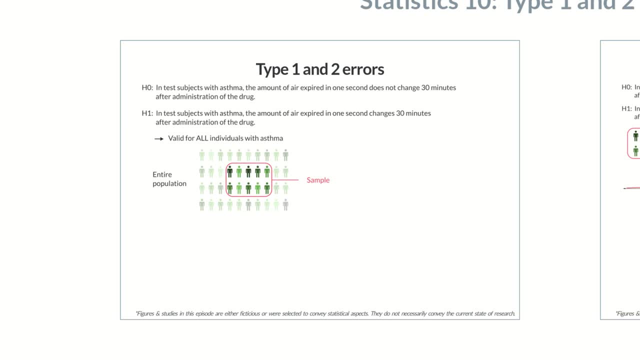 The group comprises 100 individuals with asthma who are receiving the new drug. Let's assume that the diagram shown here depicts the results of the study. They differ significantly for the individual subjects. For example, in some participants the FEV1 value decreases despite the intervention. However, in the majority of participants, 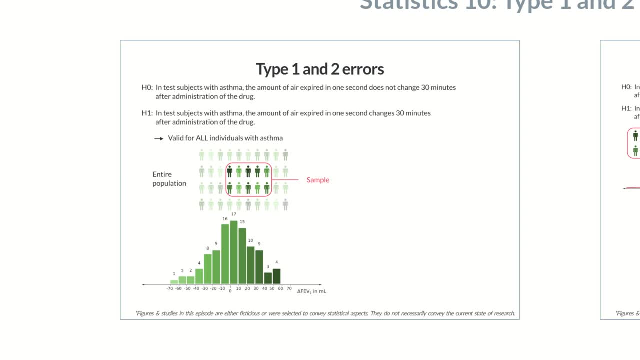 the FEV1 value improves. The data distribution can be more or less described with the bell curve. In other words, the data set here is approximately normally distributed, But that's not always the case. The mean FEV1 value improves by approximately 4 milliliters. in all participants with asthma, This corresponds to less than 1% of. 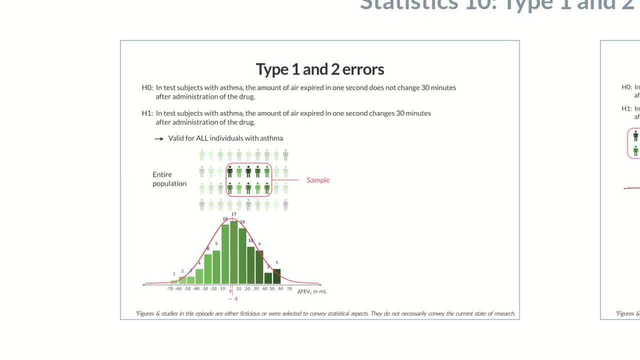 the normal tidal volume in adults. Based on this result, can the null hypothesis be rejected in favor of the alternative hypothesis? Can we state that the new drug is effective in patients with asthma If the study included the entire population of individuals with asthma? the data distribution. 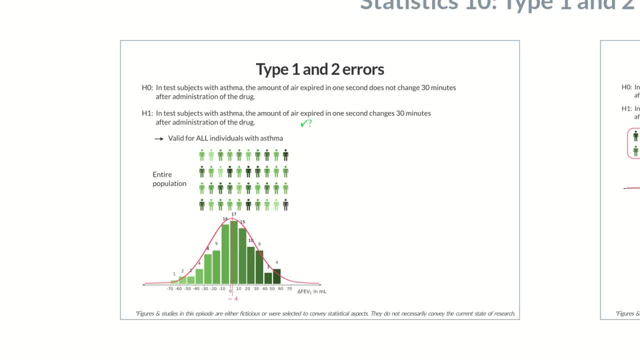 of the results would be clear and conclusive, despite the small improvement. The null hypothesis could be rejected and the alternative hypothesis accepted. But since the study only examined an exemplary representative sample of 100 participants with asthma, we need to expect room for error in the interpretation. So the question that arises is: how likely is it that the study result is due? 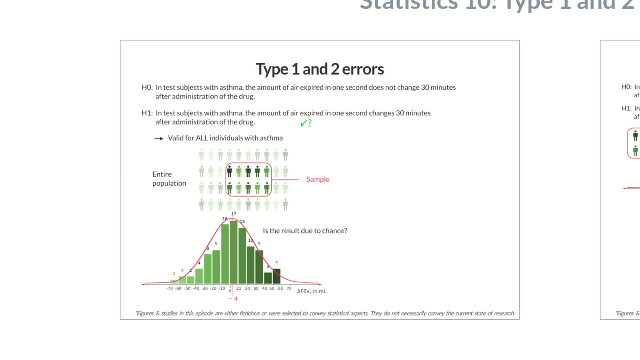 to chance, Or in other terms, how likely is this observed difference, the result When the participants on average don't actually benefit from the new drug? This question is important in assessing how certain our study result represents the real relationship. Let's suppose that we reject the null hypothesis based on our observations, even though it's actually true and 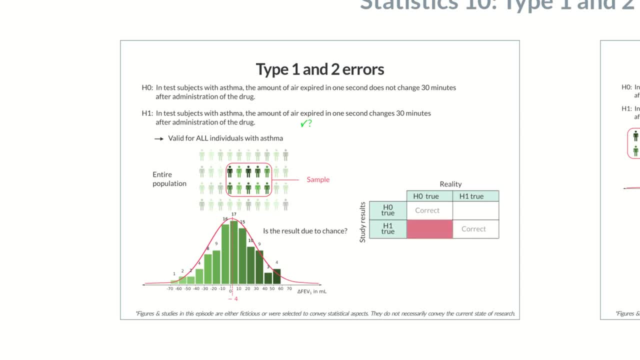 the observed results were indeed due to chance, We'd then accept a false alternative hypothesis. This is a type one error. In contrast, if we reject the alternative hypothesis even though it's true, in which case we reject the alternative hypothesis, We'd then reject the alternative hypothesis. 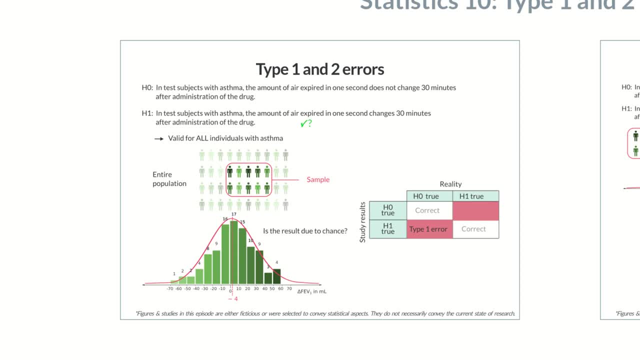 We'd then reject the alternative hypothesis even though it's true, in which case we reject the alternative hypothesis. true, that is, the null hypothesis is accepted when it's actually false. this is known as a type II error. A type I error would have large-scale implications and must be avoided. 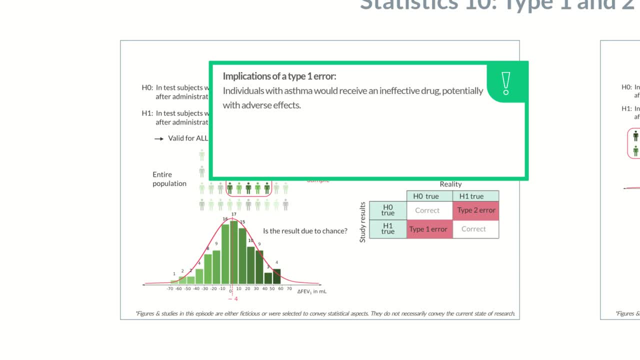 In our example, the patients with asthma would then be treated with an ineffective drug and exposed to potentially adverse effects. Also, they would miss the opportunity to be treated with another effective drug instead. However, a type II error would also have large-scale implications. 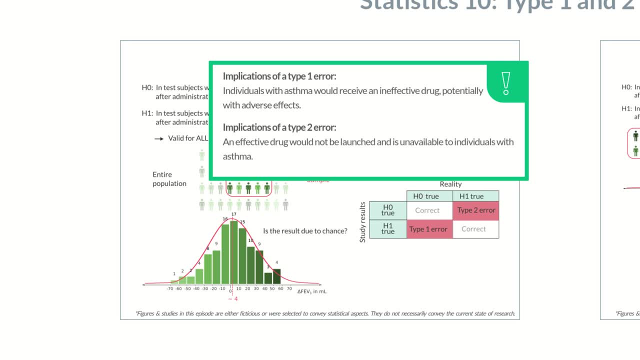 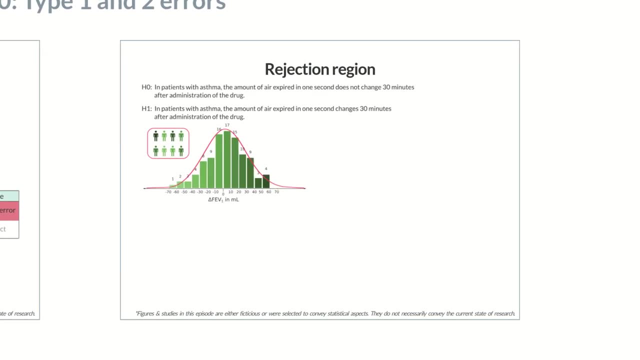 In our example, the type II error would lead to an effective drug not being launched onto the market and remain unavailable to patients with asthma. How does the knowledge of the two errors help us to interpret study data? Also, how can we assess whether the data is due to chance or reflect a true difference? 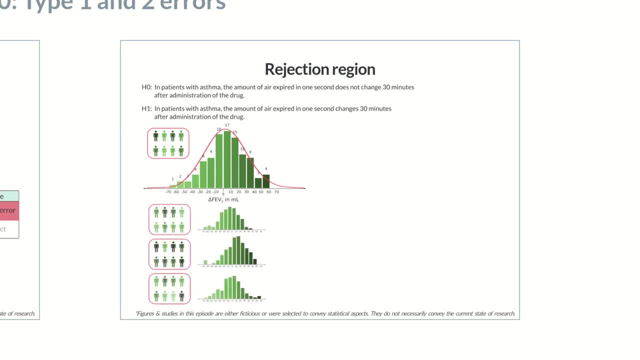 Let's take another look at our fictitious example. The average effect of the drug is 0.5.. The average effect of the drug on bronchodilation would always vary slightly when the study is conducted with different subject groups, regardless of whether the null hypothesis 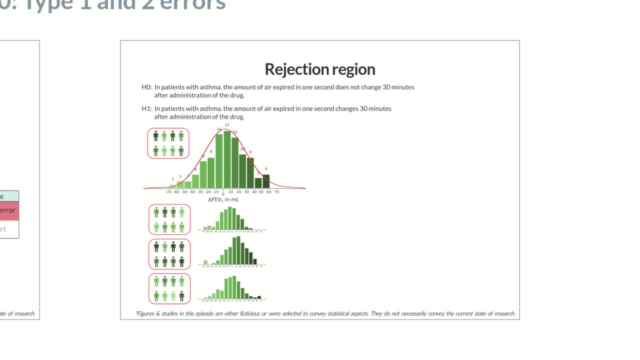 is true or false. To determine the extent of the deviation for the entire population of asthmatics, we'd need to calculate a statistical mean from the experimental mean values of the different sample groups. Assuming that the null hypothesis is true, these mean values are distributed around zero. 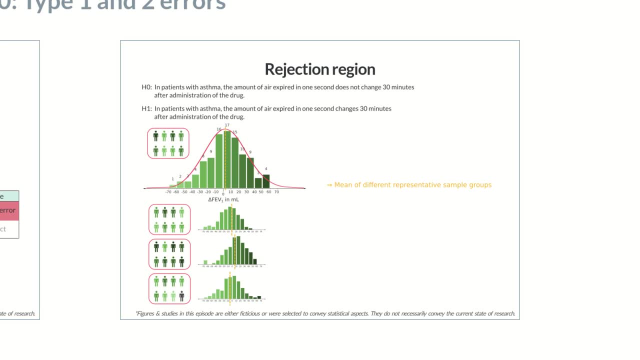 But is 4 milliliters considered close to zero or distant? No, The calculated mean value can help to examine the extent to which the drug's effect in the study reflects the mean for the entire population. The distribution of the mean values for the entire population would produce a bell curve. 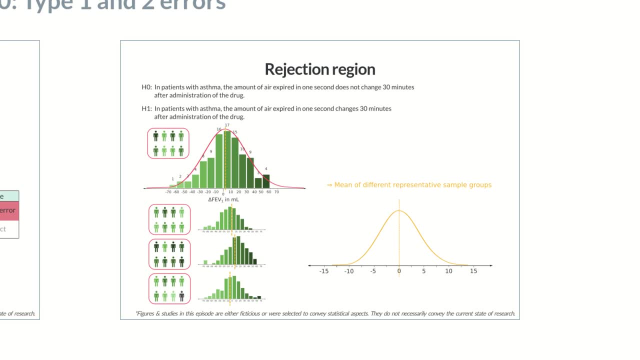 In practice. repeating studies is too time-consuming and expensive. So from the mean and scatter of the study data we can theoretically determine how large the probability is to reject a true null hypothesis. The type 1 error is defined by the study design. 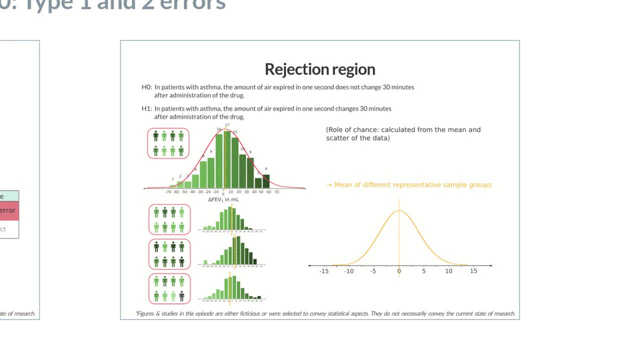 In medical research, the type 1 error rate, also called the significance level, or simply denoted with alpha, is usually set to 5%. If a one-tailed test is performed, this 5% lie on the side of the curve whose range of 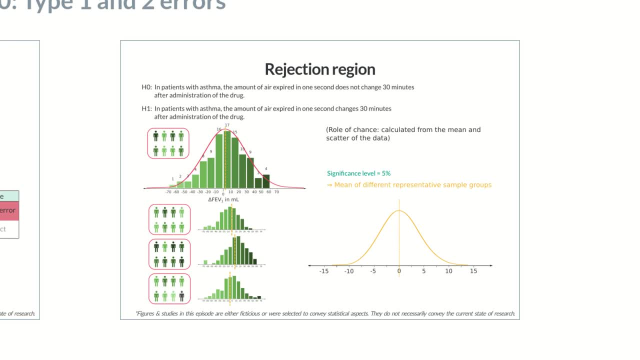 values is examined. In contrast, if a two-tailed test is performed, the 5% are split. The difference between the two-tailed test and the one-tailed test is that the two-tailed test is the one-tailed test.